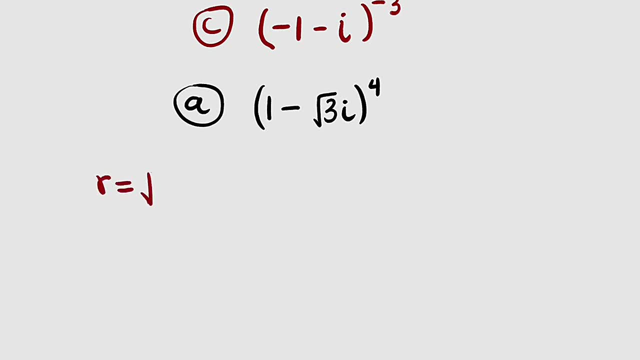 So we have r equal to the square root of what Real part squared, and the real part is 1 squared. then, plus the imaginary part, which is negative root, 3 also squared. 1 squared is 1.. Negative root: 3 squared is just 3.. 1 plus 3 is 4.. Square root of 4 is 2.. Remember that. 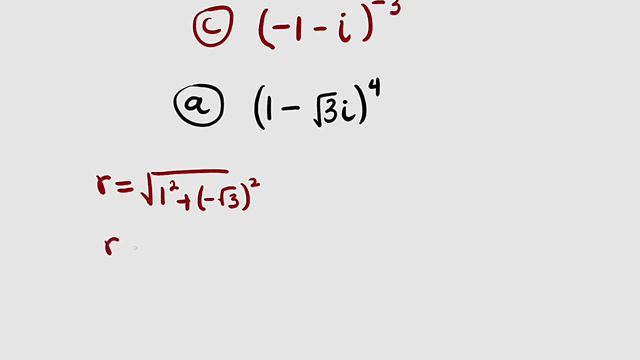 r is a modulus, which is a distance right. So we are going to write the positive solution. This is what only true. Then what about the angle subtended? If you observe, this is in the fourth quadrant right. That is where the real part is positive and the imaginary part is negative. 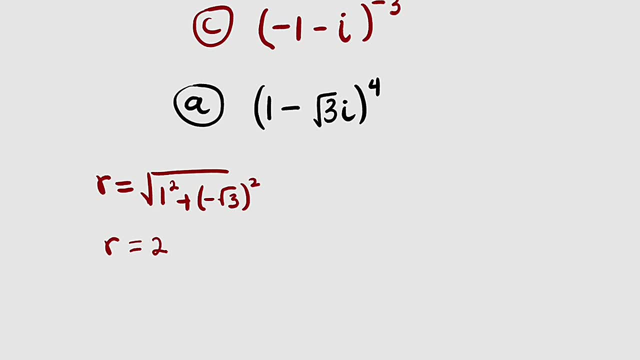 But we are going to assume we are in the first quadrant because walking in the first quadrant is very simple. But in the end, since we are in the third quadrant, we are going to subtract the result from 360 degrees. So remember that Our reference angle in the first quadrant will be equal to tan inverse of only the positive. 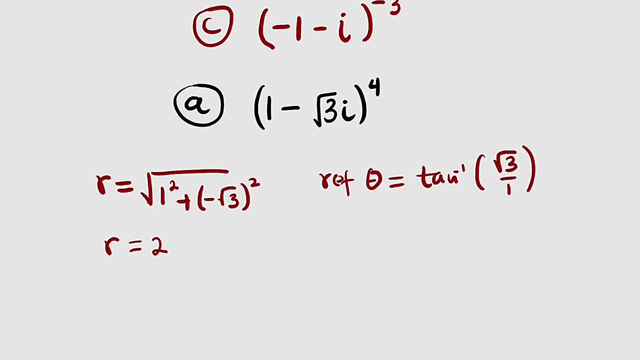 values. root 3 divided by 1. Root 3 divided by 1 is root 3, and tan inverse of root 3 is 60 degrees, or pi divided by 3.. So therefore this is equal to pi divided by 3.. But our 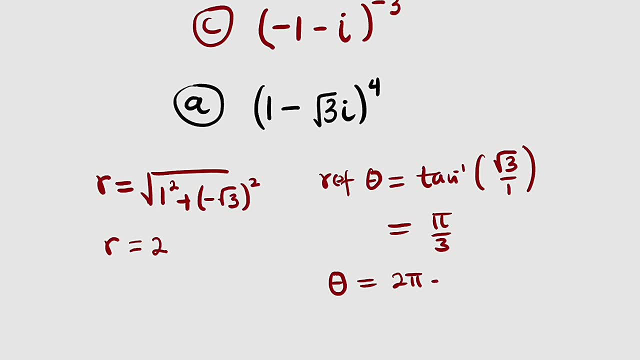 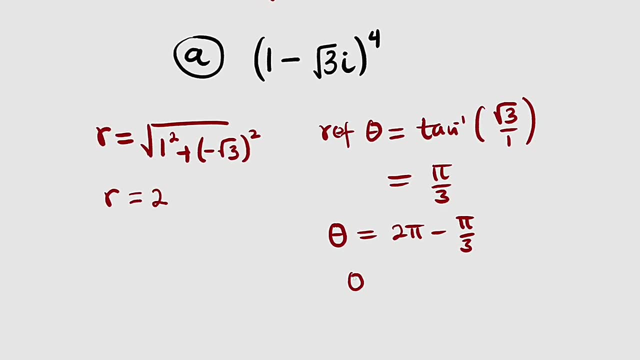 main angle, theta will be equal to 2 pi minus pi divided by 3., Which is equal to 5 pi divided by 3 right. So the angle is equal to 5 pi divided by 3.. So, having obtained the radius and the angle, we can now write this complex number in polar form. 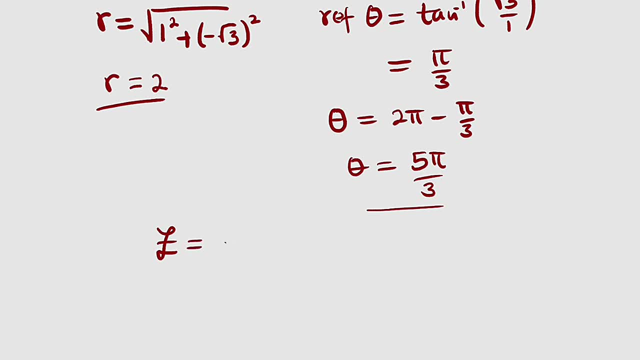 So our z, equal to r, which is 2, multiplied by cosine of that angle, which is 5 pi divided by 3.. Then plus i, multiplied by sine of the same angle: 5 pi divided by 3.. But remember, we are looking for z to which power? To the power of 4.. 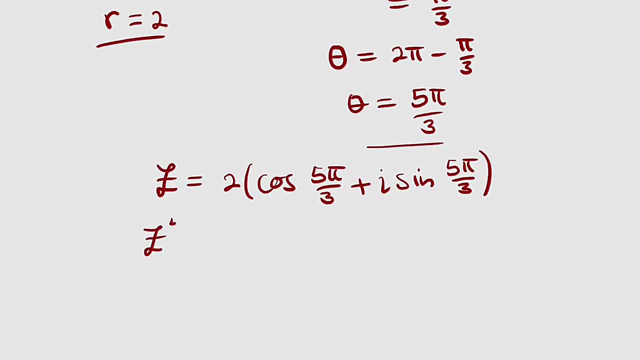 Therefore, we are going to raise this to the power of 4.. z to the power of 4 will be equal to 2 to the power of 4 multiplied by cosine of this angle multiplied by 4.. If you multiply it by 4, you have: 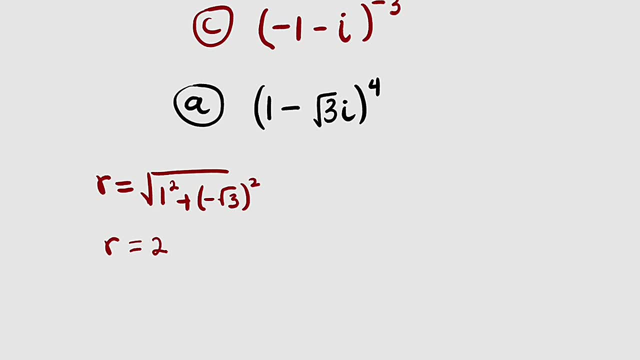 But we are going to assume we are in the first quadrant because walking in the first quadrant is very simple. But in the end, since we are in the third quadrant, we are going to subtract the result from 360 degrees. So remember that Our reference angle in the first quadrant will be equal to tan inverse of only the positive. 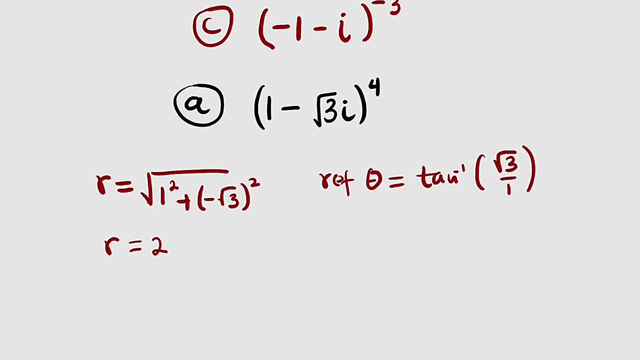 values. root 3 divided by 1. Root 3 divided by 1 is root 3, and tan inverse of root 3 is 60 degrees, or pi divided by 3.. So therefore this is equal to pi divided by 3.. But our 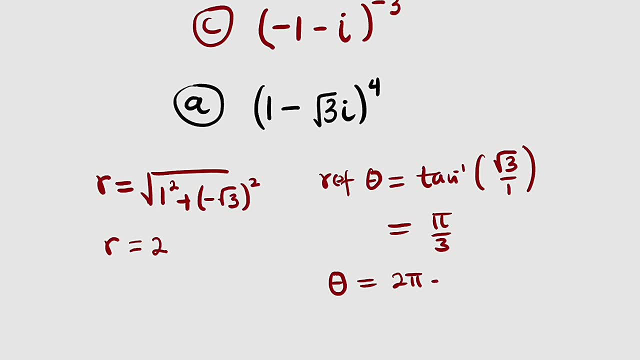 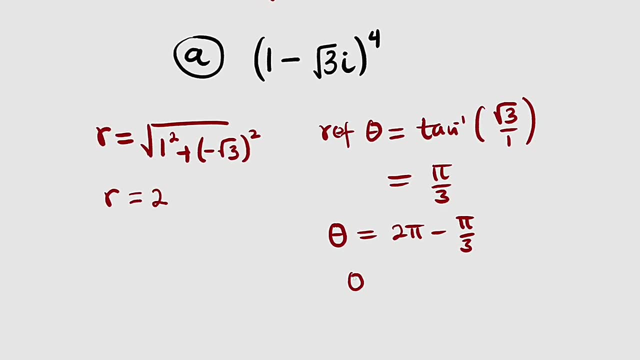 main angle, theta will be equal to 2 pi minus pi divided by 3., Which is equal to 5 pi divided by 3 right. So the angle is equal to 5 pi divided by 3.. So, having obtained the radius and the angle, we can now write this complex number in polar form. 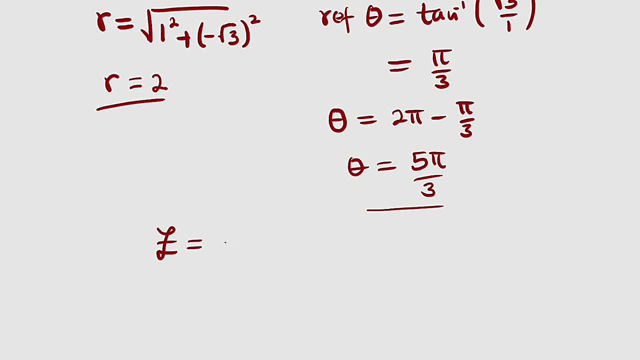 So our z, equal to r, which is 2, multiplied by cosine of that angle, which is 5 pi divided by 3.. Then plus i, multiplied by sine of the same angle: 5 pi divided by 3.. But remember, we are looking for z to which power? To the power of 4.. 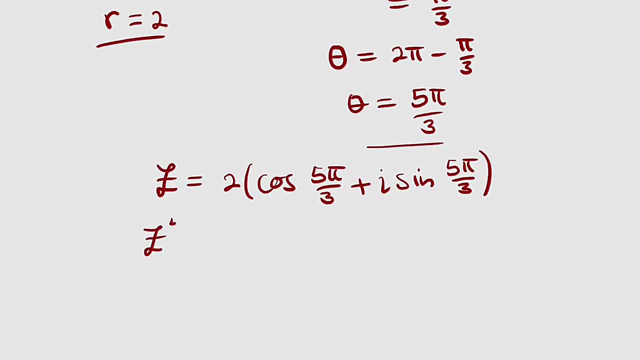 Therefore, we are going to raise this to the power of 4.. z to the power of 4 will be equal to 2 to the power of 4 multiplied by cosine of this angle multiplied by 4.. If you multiply it by 4, you have: 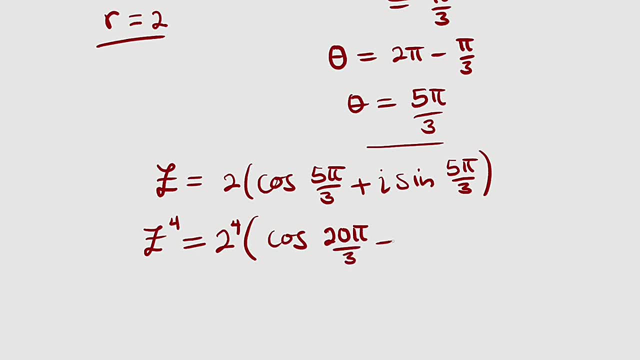 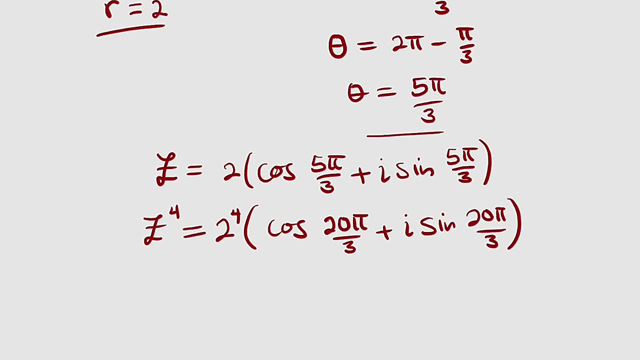 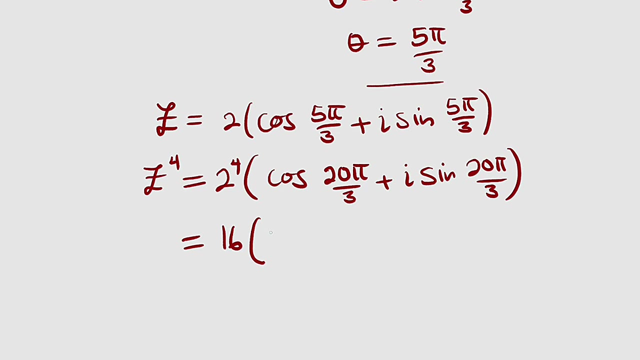 20 pi divided by 3, plus i sine of 20 pi divided by 3.. So this is equal to 2 pi divided by 3.. This is equal to 2 to the power of 4 is 16.. And cosine of 20 pi divided by 3 is equal. 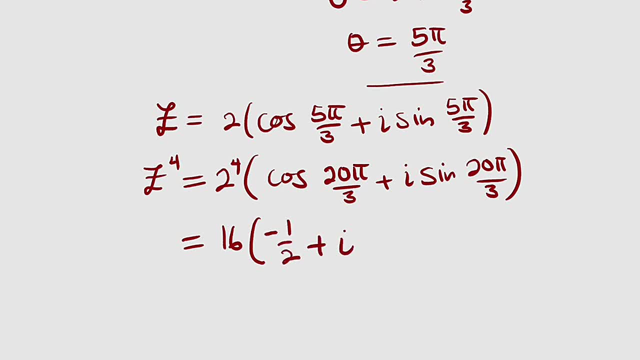 to negative 1 divided by 2.. Then plus i multiplied by sine of 20 pi divided by 3.. And sine of 20 pi divided by 3 is root 3 divided by 2.. So we have root 3 divided by 2.. So this is. 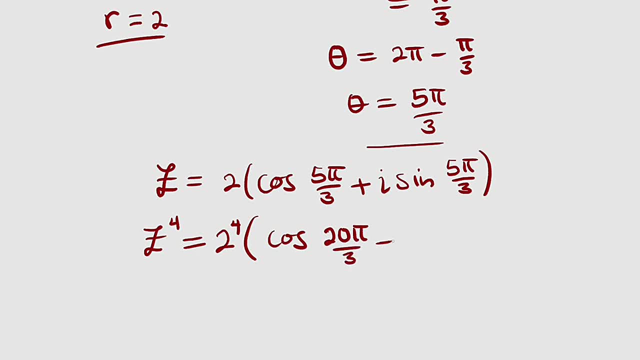 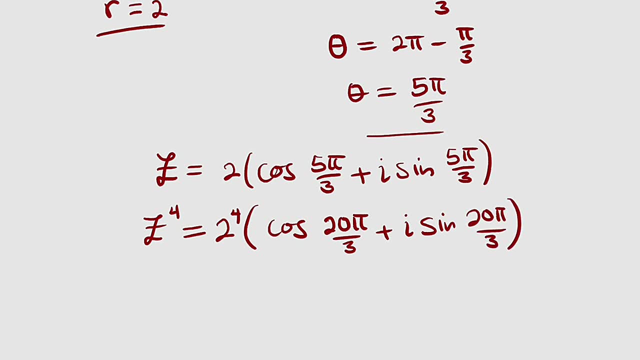 20 pi divided by 3 plus i sine of 20.. So sine of 2 to the power of 4.. 3 pi divided by 3.. Therefore, this equal to 2 to the power, 4 equal to 16.. Then we will put this and connect this to the right position. 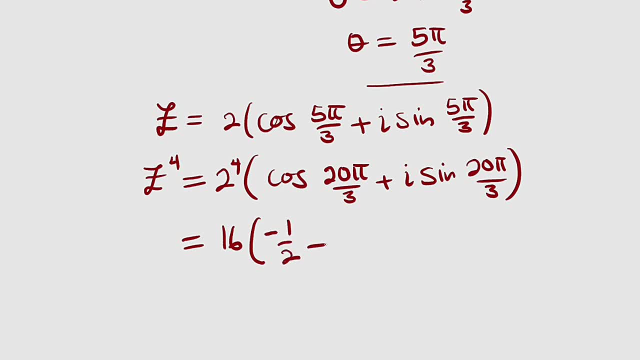 Then we have cosine of 20 pi divided by 3, plus i times the sine of 20 pi divided by 3.. And then we have cosine of 2 to the power 4 equal 2 pi into it equals 2 pi divided by 2.. 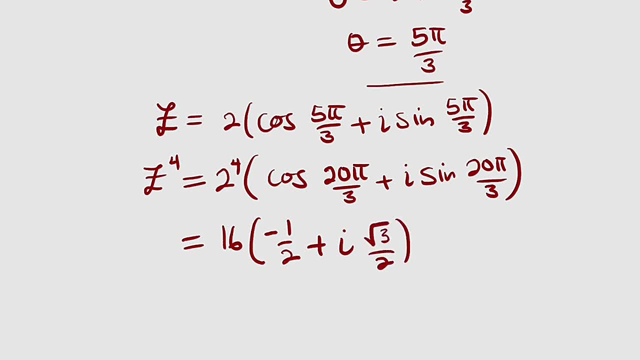 So we87d the power of 4 to the power of 4 equals 16.. And so cos of 20p真的很 numerical- to negative 1 divided by 2.. And then the hand accordance is negative 1 divided by 2.. plus i multiplied by sine of 20 pi divided by 3.. And 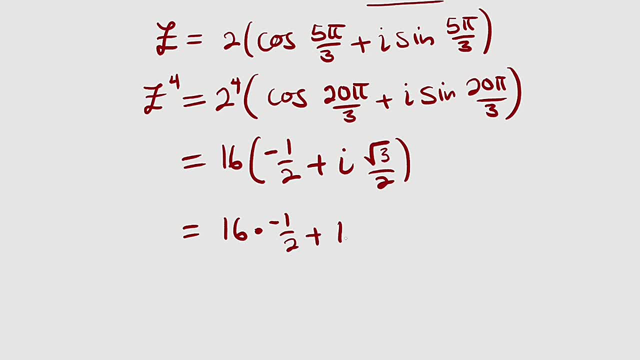 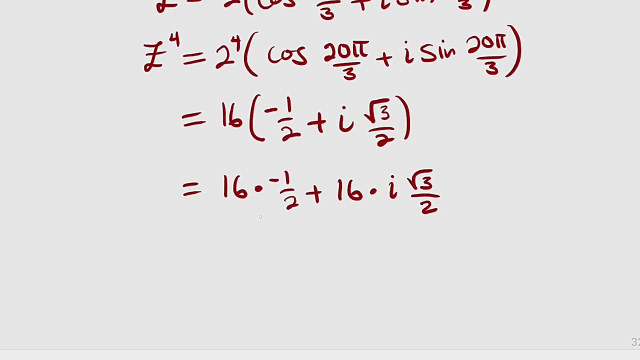 multiplied by negative, 1 over 2, plus 16, multiplied by i root, 3 divided by 2. 2 will go into 16: 8 times. so we have negative 8 here, plus 2 will go into 16: 8 times, so we have: 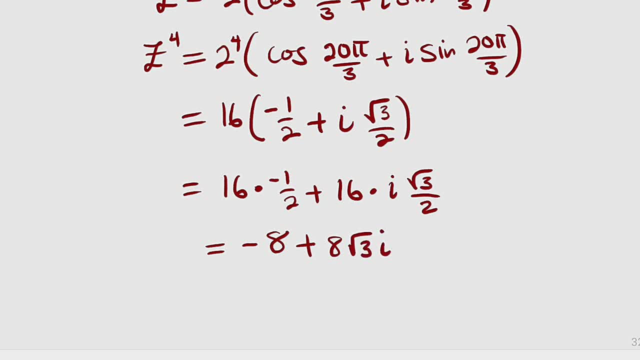 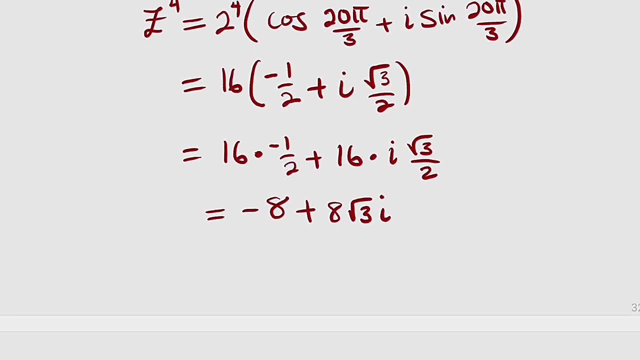 8 root 3 i. So if you expand this complex number, 1 minus root 3 i, to the power of 4, you're going to obtain negative 8 plus 8 root 3 i. So now let us move on to the second problem. 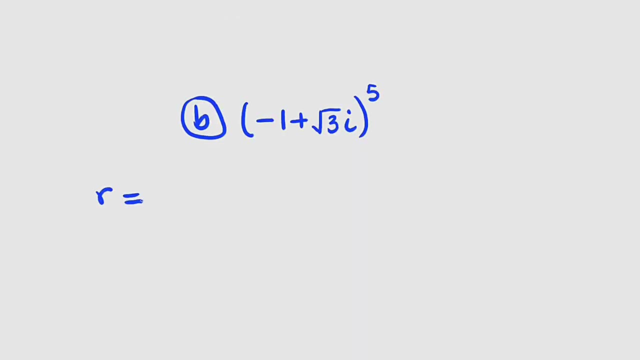 First of all, let us find r, which is the modulus. r will be equal to the square root of real part squared, plus the imaginary part also squared. Without wasting time, this is equal to 2.. Then what about the angle? If you observe, this is in the second quadrant, right, which is less. 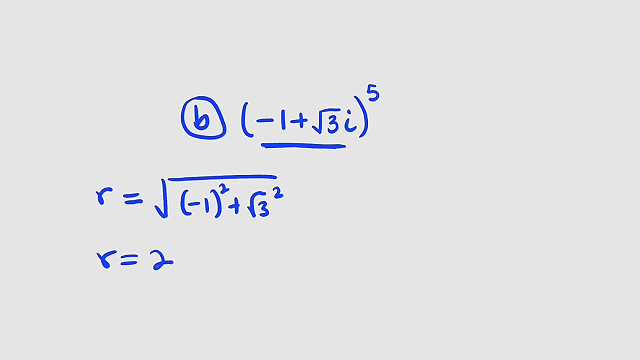 than 100.. So we are going to use first quadrant as reference, but whatever we obtain, we have to take it away from 180 degrees or pi, because we are in the second quadrant. So reference theta is equal to tan inverse of what Root 3 divided by 1.. 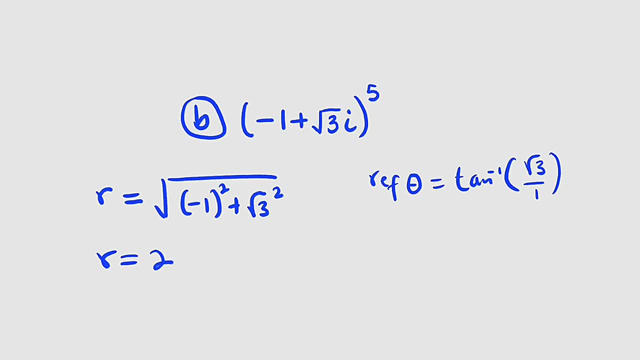 And root 3 divided by 1 is root 3.. Tan inverse of root 3 is equal to 60 degrees, or pi divided by 3.. So therefore, this is pi divided by 3.. But remember we are in the second quadrant. 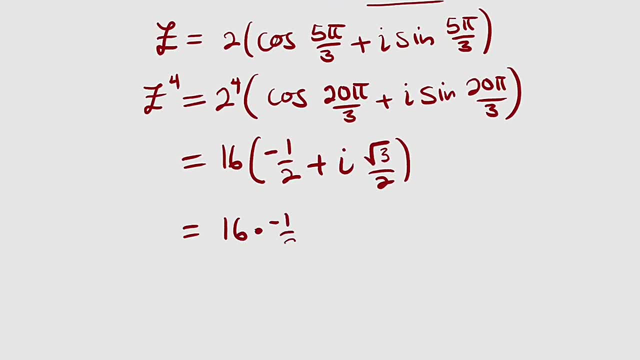 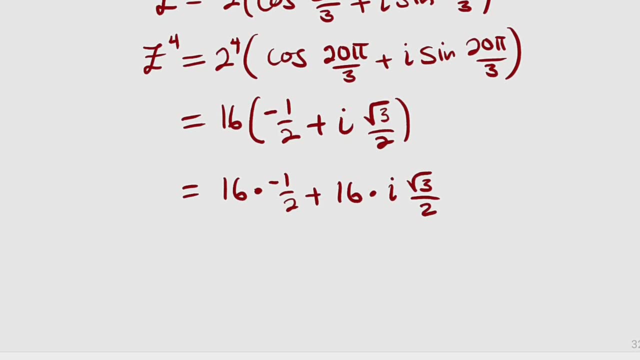 equal to 16 multiplied by negative 1 over 2, plus 16 multiplied by i root 3, divided by 2.. 2 will go into 16, 8 times, so we have negative 8 here, Plus 2 will go into 16: 8 times, so we have 8 by root 3 i. So if you expand it, from this complex number 1 minus root 3 i to the power of 4, you're going to obtain two complex numbers: 1 minus root 3 I to the power of 4, you're going to obtain two complex numbers. First of all, remember: if you then add all of the components, then again you get less than. 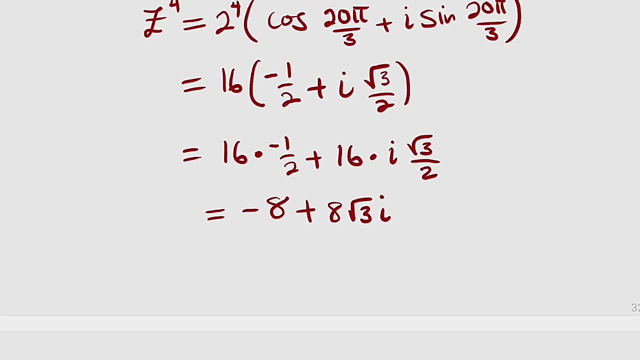 1 right right Once. if you You Bye now. so that means we're done, even though we did another card here. So now what do we have before? this is 2 plus 1 minus root 3 I by root Negative 8 plus 8 root 3i. 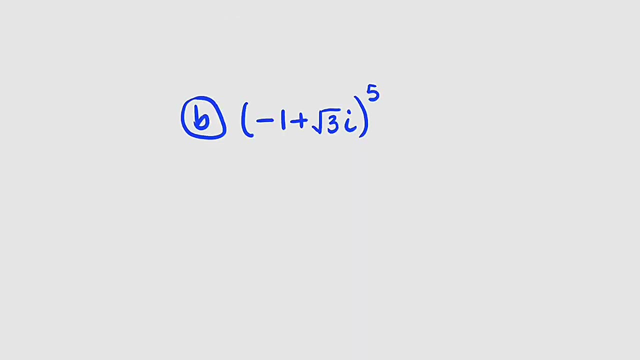 So now let us move on to the second problem. First of all, let us find r, which is the modulus. r will be equal to the square root of real part squared, plus the imaginary part also squared. Without wasting time, this is equal to 2.. 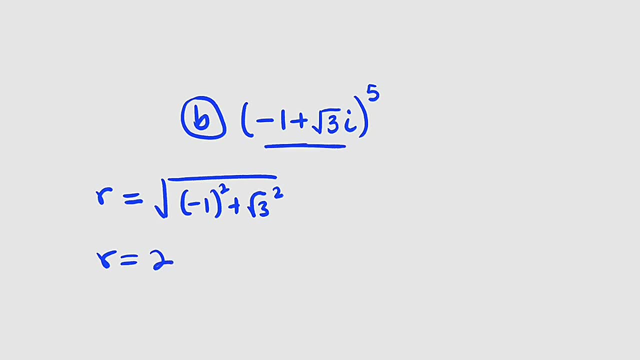 Now, what about the angle? If you observe, this is in the second quadrant, right, which is less than 180 degrees. So we are going to use first quadrant as reference, But whatever we obtain, we have to take it away from 180 degrees or pi, because we are in the second quadrant. 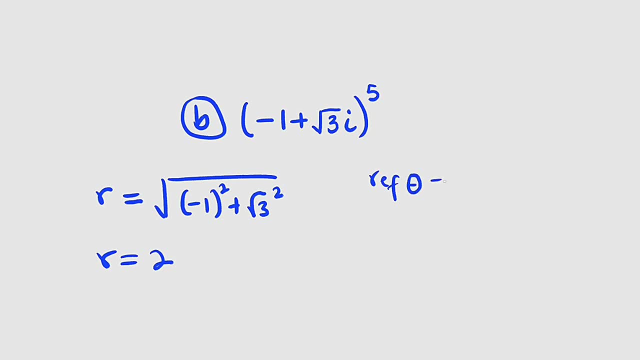 So reference theta is equal to tan inverse of what Root 3 divided by 1.. And root 3 divided by 1 is root 3.. Tan inverse of root 3 is equal to 60 degrees, or pi divided by 3.. 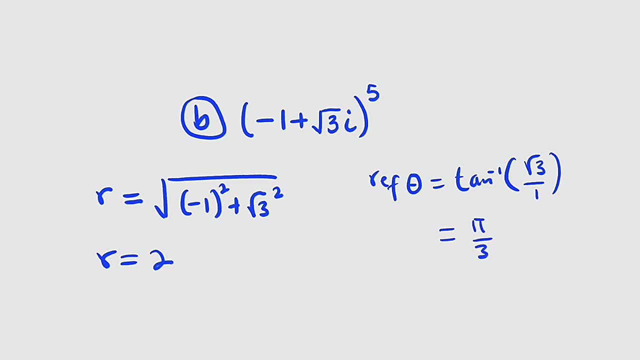 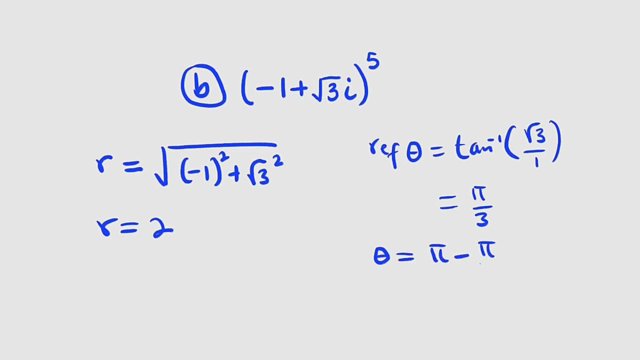 So therefore, this is pi Divide by 3.. But remember we are in the second quadrant. Therefore our main theta will be equal to pi minus pi divided by 3, which is equal to what 2pi divided by 3.. 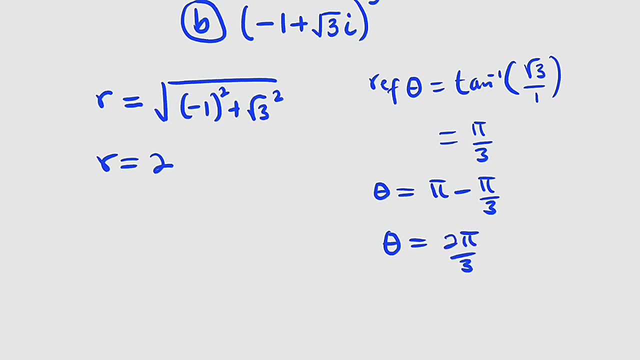 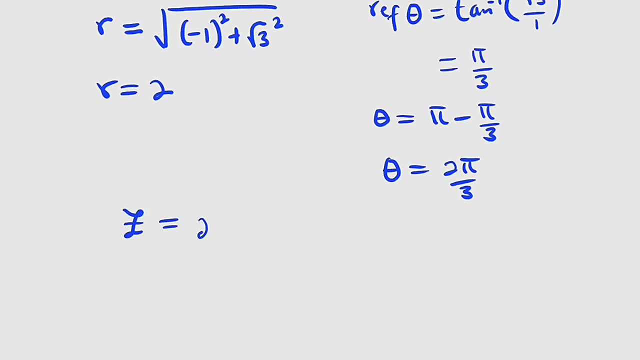 Theta is now equal to 2pi divided by 3.. So our complex number in polar form, z, is equal to the radius, which is 2.. Then multiply by cosine of that angle: 2pi Divide by 3.. Then plus i, sine of what? 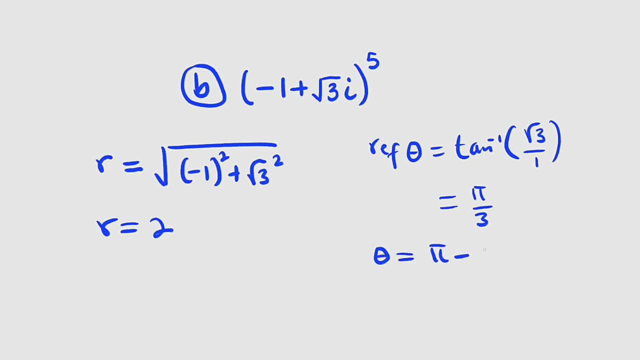 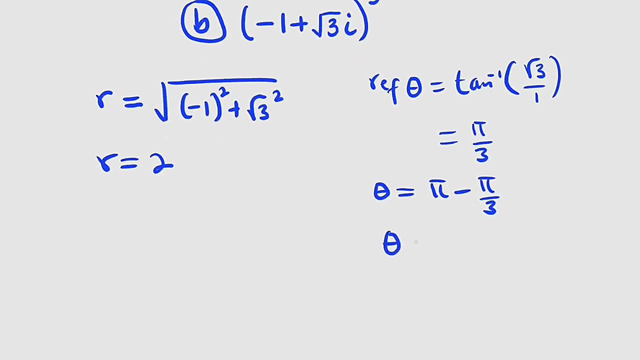 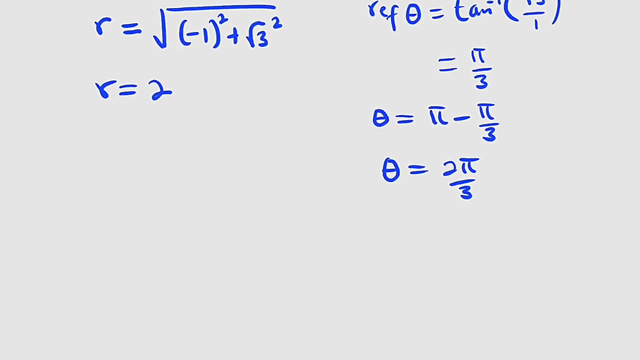 Therefore our main theta will be equal to pi minus pi divided by 3, which is equal to what 2 pi divided by 3.. Theta is now equal to 2 pi divided by 3.. So our complex number in polar form, z, is equal to the radius, which is 2.. Then multiply by cosine of that. 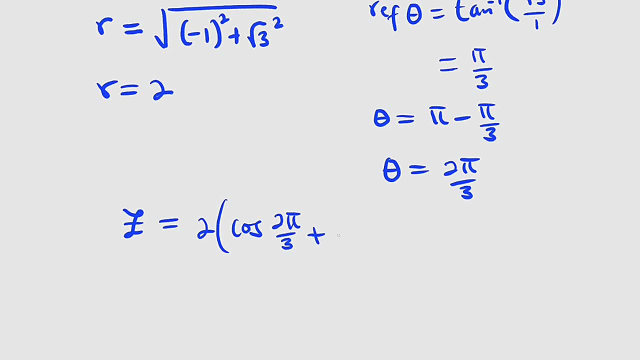 sei equals to r, capable of bigger or less than 7 times the ratio of pi divided by 3.. enorme equal to r. screen DESCHriM. Now the w is the last answer, Then, what we are looking for? this complex number z is equal to z, to the power of. 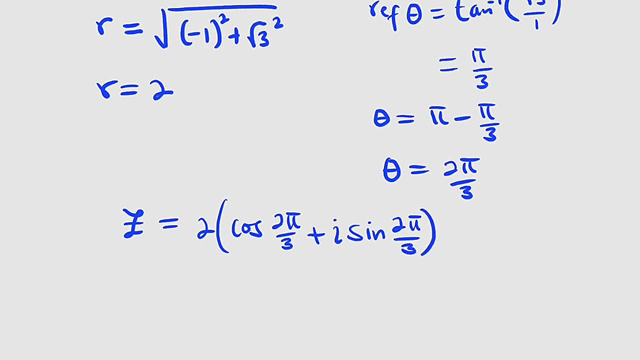 n equal to 1 total times one. n equal to oriented hyperbolic angle, 2 pi divided by 3.. but we are looking for this complex number, to which power? to the power of 5.. And we can say, for real, we have the two es mistake. 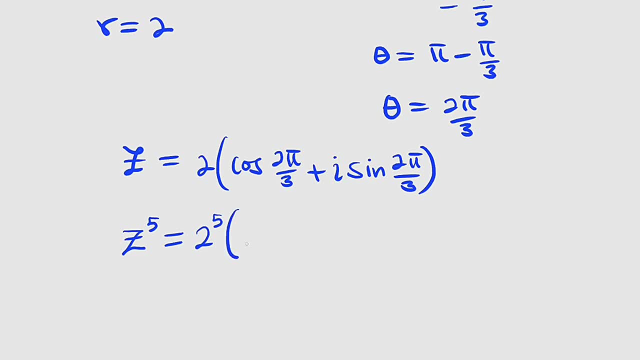 So z is equal to two devices on the fourth planet. So here see dream equation: two of r equals n equals t in the external о, x is equal to the power of r plus times a, the original zero over pi divided by degrees. we can also use a one statement-based怎樣 and add into this equation. 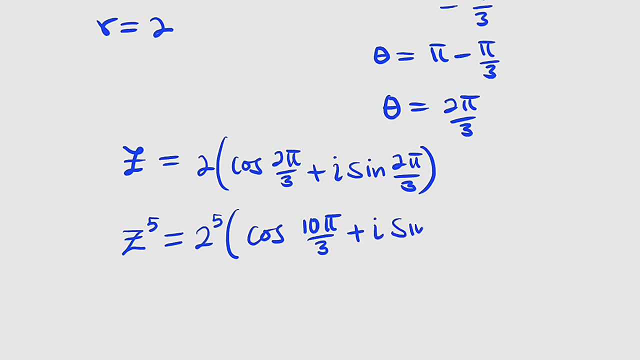 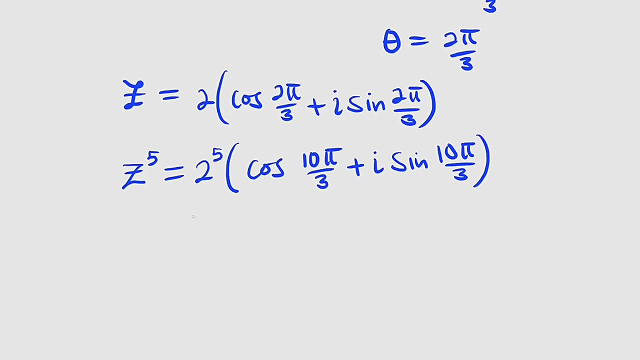 The function of alpha equals the cube square honor pi squared by zero. then plus i sine of what? 10 pi divided by 3.. 2 to the power of 5 is 32.. So this is equal to 32 multiplied by the whole of this Cosine of 10 pi divided by 3 is negative 1 divided by 2.. 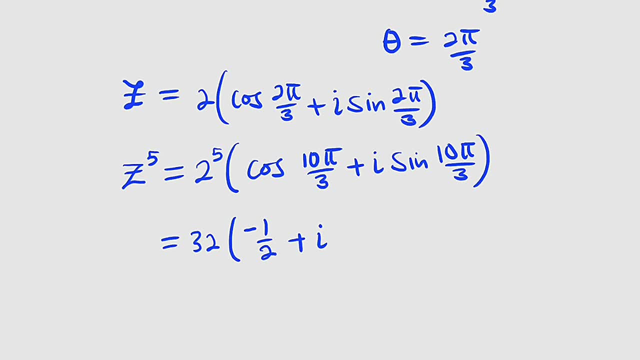 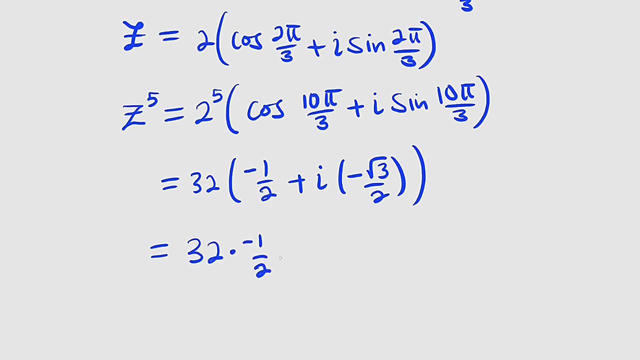 Then plus i multiplied by sine of the same angle, which is negative root 3 divided by 2.. So now let us expand. This is the same thing as 32 multiplied by negative 1 divided by 2, plus i, 32 multiplied by what? Negative root 3 divided by 2.. 2 will go into 32, 16 times 16. 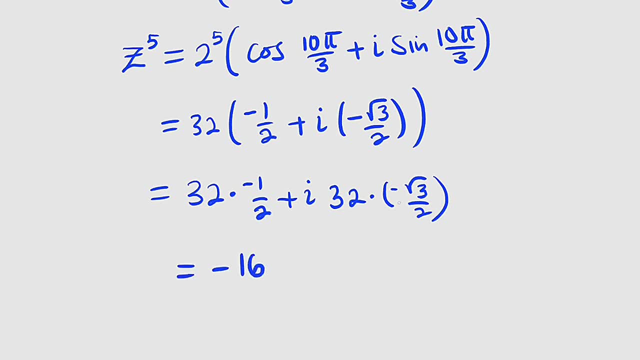 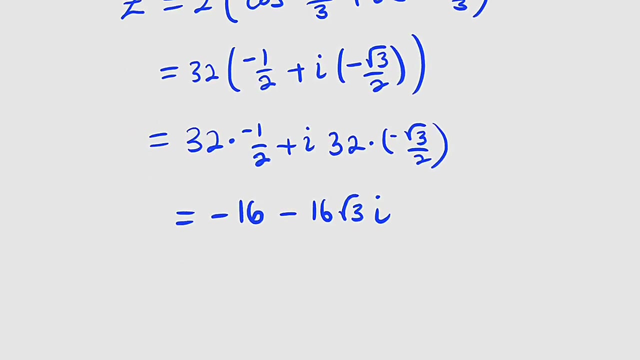 times negative 1. This is equal to negative 16. This is also negative, So we have negative 16 root 3.. So this implies that if you expand this complex number to the power of 5, you're going to obtain negative 16- negative 16 root 3- i. If you like, you can use your calculator to expand this to. 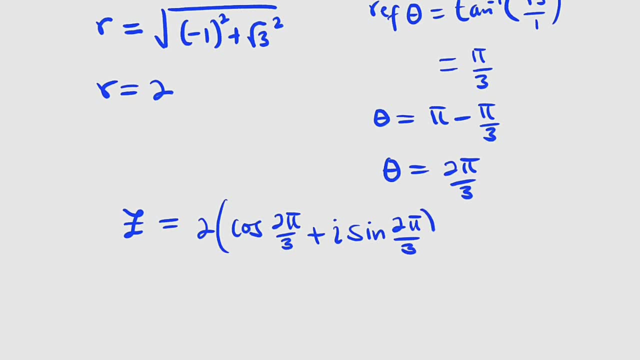 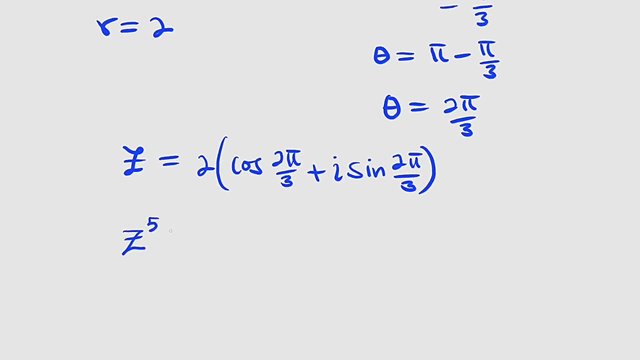 The same angle: 2pi divided by 3.. But we are looking for this complex number to which power, To the power of 5.. So z to the power of 5 is equal to 2 to the power of 5 multiplied by cosine of 5, multiplied by this angle, which is 10pi divided by 3, right. 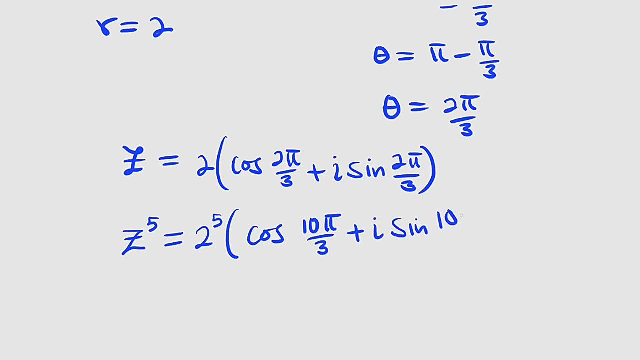 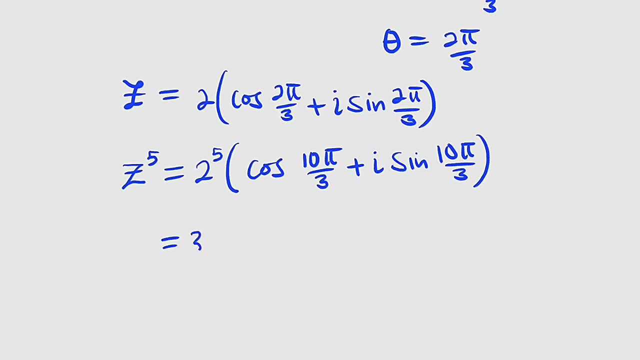 Then plus i sine of Of what: 10pi divided by 3.. 2 to the power of 5 is 32.. So this is equal to 32.. Multiply by the whole of this Cosine of 10pi divided by 3 is negative 1 divided by 2.. 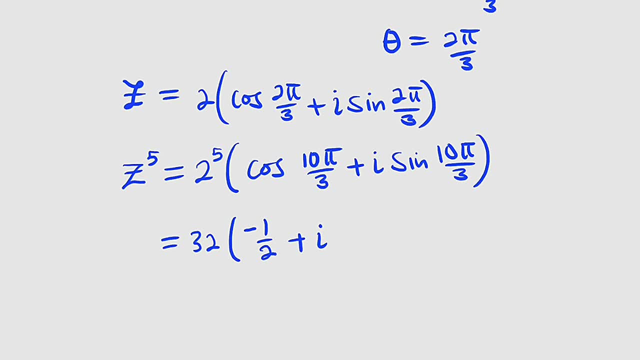 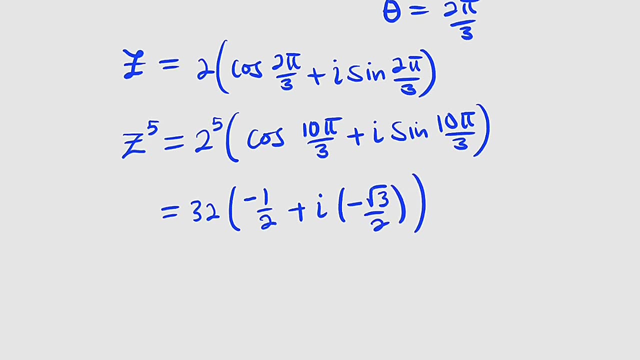 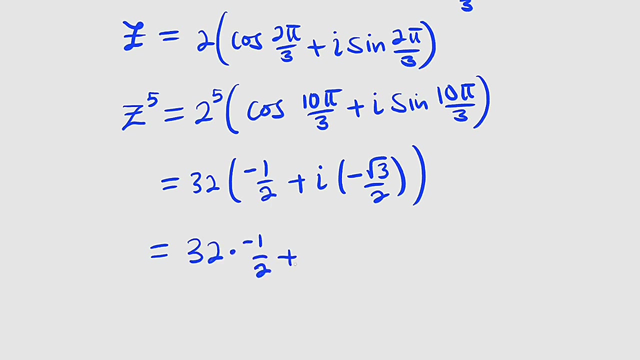 Then plus i, multiplied by sine of the same angle, which is negative root, 3 divided by 2.. So now let us expand. This is the same thing, That's 32 multiplied by negative, 1 divided by 2, plus i, 32, multiplied by what? 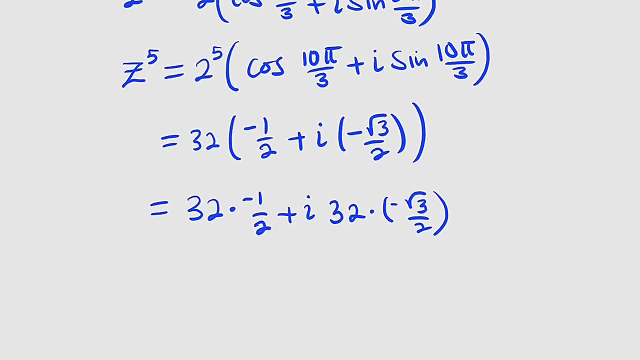 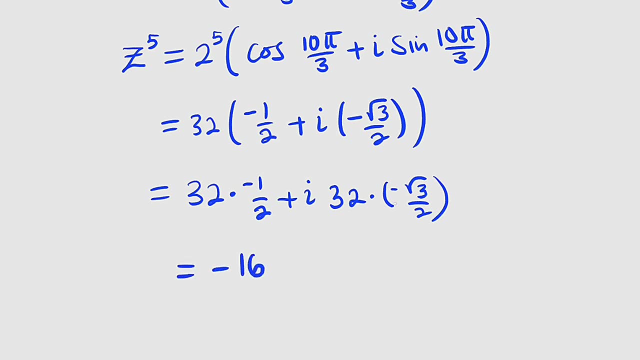 Negative root 3 divided by 2.. 2 will go into 32, 16 times, 16 times negative 1. This is equal to negative 16. This is also negative. So we have negative 16 root 3i. 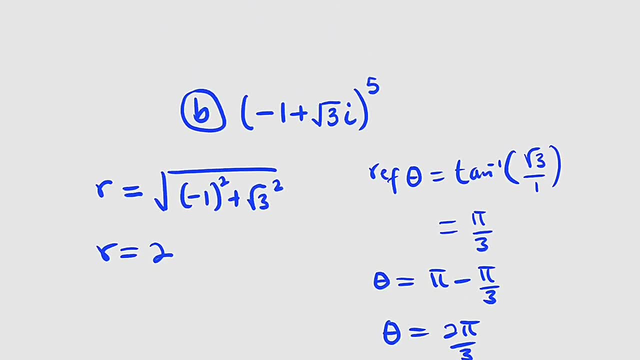 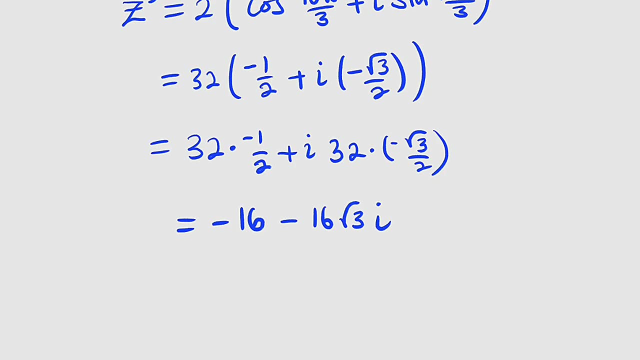 So this implies that if you expand this complex, this complex number to the power of 5, you're going to obtain negative 16, negative 16 root 3i. If you like, you can use your calculator to expand this to see whether this is true. 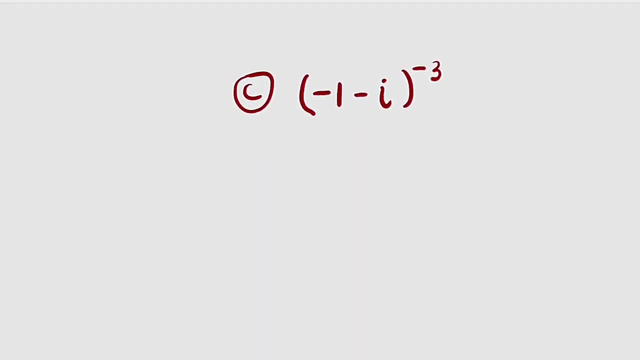 So now let us take the last question. Here is our last question. We have negative 1, negative i, but to the power of negative 3. So we can rearrange this as 1 divided by negative 1, negative i. 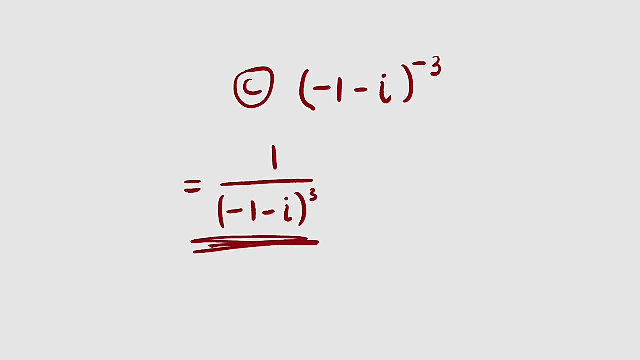 to the power of 3.. So this is what we need: to expand first, then we bring it back here, rationalize and get our final result. So what will be our radius Will be what Square root of negative 1 squared plus negative 1, also squared? 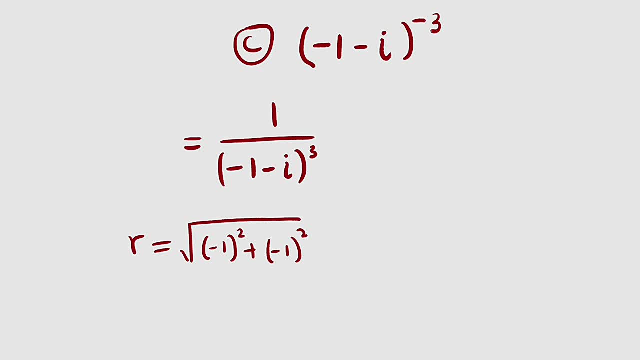 because the coefficient of i is negative, 1.. Negative 1 squared is 1.. 1 plus 1 is 2.. So we have square root of 2. here r is equal to Square root of 2.. So what about the angle? 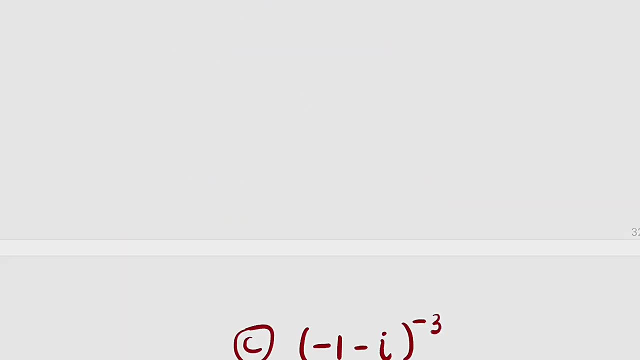 see whether this is true. So now let us take the last question. Here is our last question. We have negative 1, negative i, but to the power of negative 3.. So we can rearrange this as negative 1, negative i to the power of 3.. So this is what we need to expand first, Then we bring it. 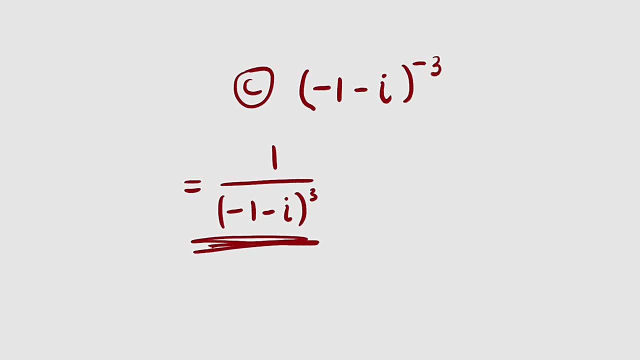 back here, rationalize and get our final result. So what will be our radius? It will be what Square root of negative 1 squared plus negative 1 also squared, because the coefficient of i is negative 1.. Negative 1 squared is 1.. 1 plus 1 is 2.. So we have square root of negative 1 squared. 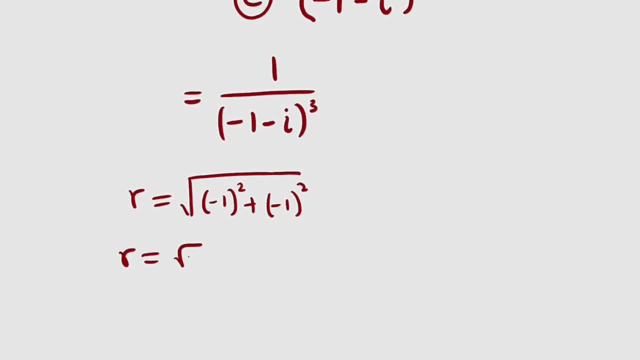 Square root of 2. here r is equal to square root of 2.. So what about the angle? If you observe, this is in the third quadrant, which is greater than 180.. So we are going to use first quadrant as reference, But whatever we obtain, we have to add it to 180 o pi. So theta reference. 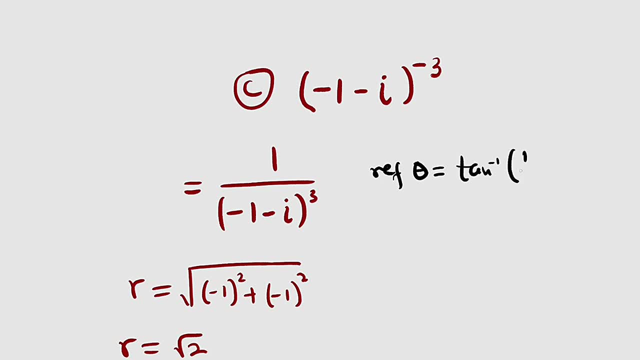 is equal to what Tan inverse of 1 divided by 1.. That is imaginary part divided by the real part. 1 divided by 1 is 1.. So tan inverse of 1 is equal to 45 degrees. But remember we are in the third quadrant, Therefore our main theta will be equal. 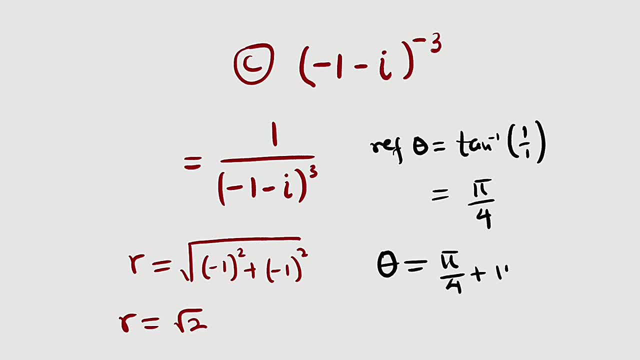 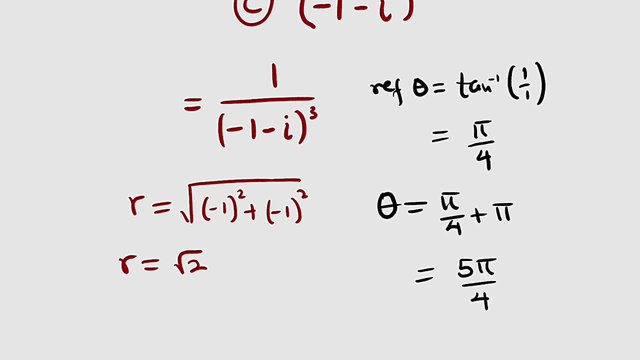 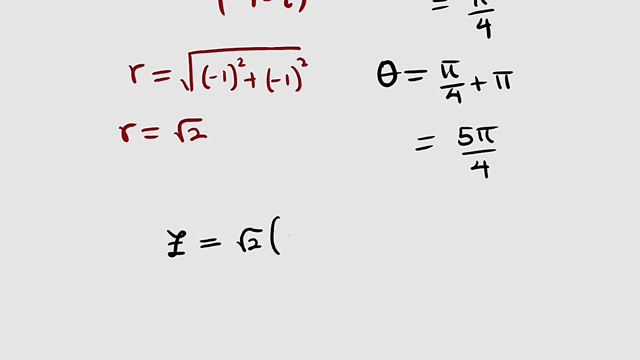 to pi divided by 4, then plus pi, And this will give us what 5 pi divided by 4.. Therefore our complex number z will be equal to r. Then multiply by cosine of what 5 pi divided by 4, plus i sine 5 pi divided by 4.. But we are looking. 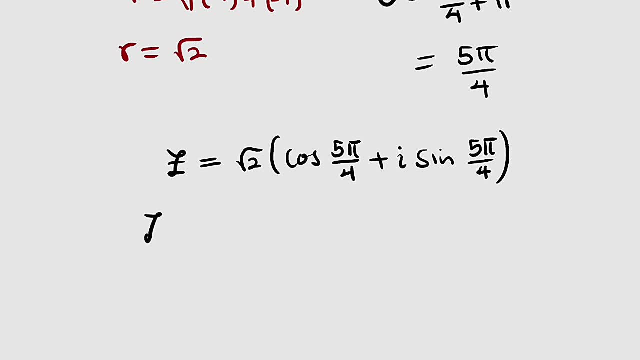 for this complex number to the power of 3.. So we have z to the power of 3, which is equal to root 2 to the power of 3 multiplied by cosine of what 15.. 5 pi divided by 4.. If you multiply that by 3, then plus i sine of what 15 pi divided by 3.. 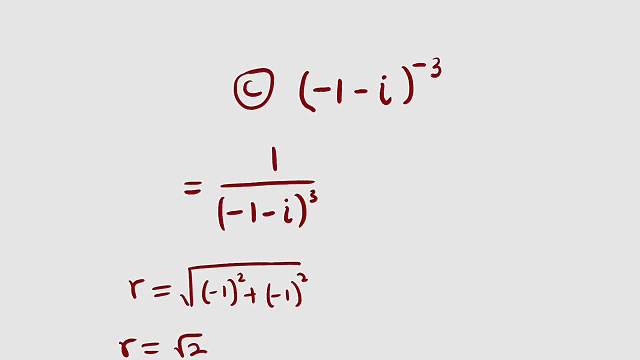 If you observe, this is in the third quadrant, which is greater than 180. So we are going to use first quadrant as reference, but whatever we obtain, we have to add it to 180, or pi, So theta reference is equal to what? 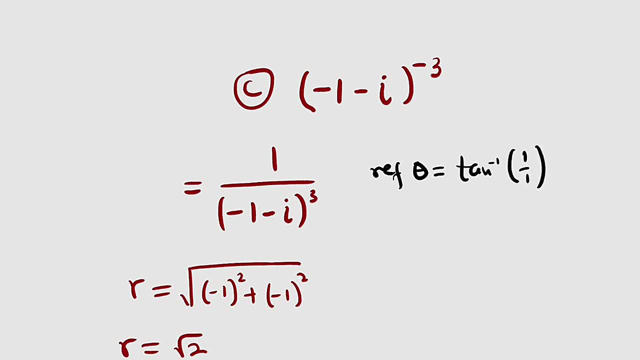 Tan inverse of 1 divided by 1.. That is imaginary part divided by the real part. 1 divided by 1.. 1 is 1.. So tan inverse of 1 is equal to 45 degrees. But remember we are in the third quadrant. 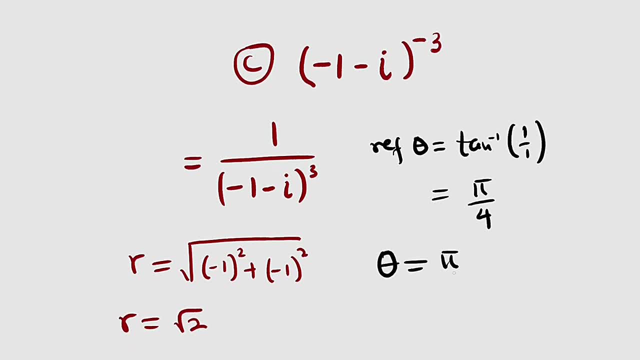 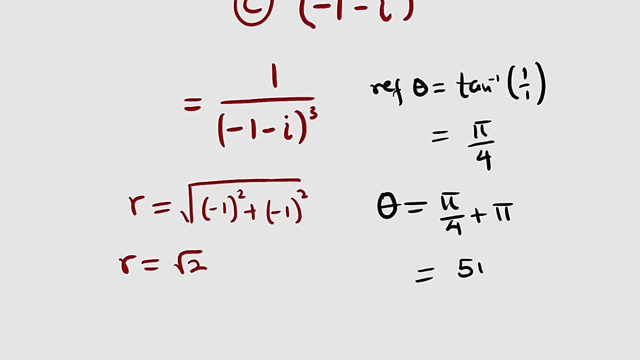 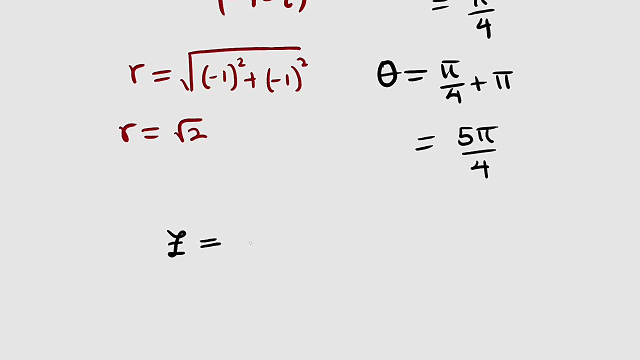 Therefore our main theta will be equal to pi divided by 4, then plus pi, And this will give us what 5 pi divided by 4.. Therefore our complex number z will be equal to r. Then multiply by cosine. 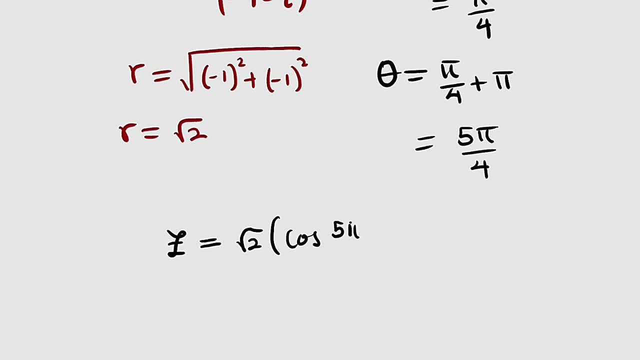 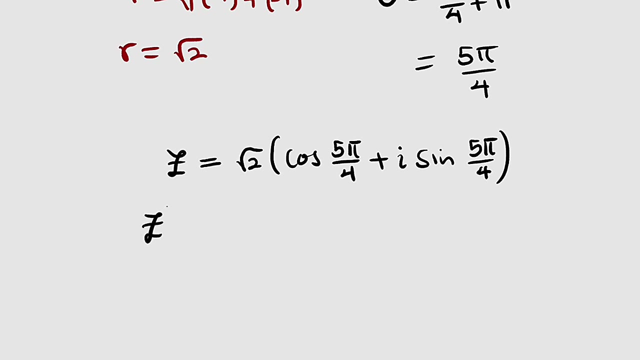 Multiply by cosine of what: 5 pi divided by 4 plus i sine 5 pi divided by 4.. When we are looking for this complex number to the power of 3, so we have z to the power of 3, which is equal to root 2 to the power of 3 multiplied by cosine of what. 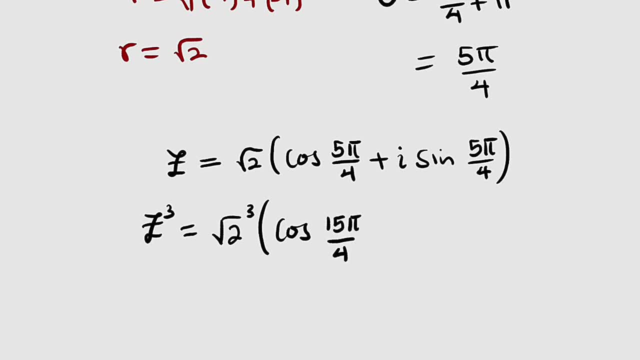 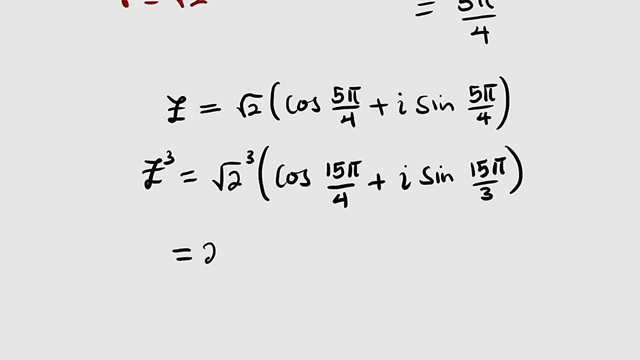 15 pi divided by 4.. If you multiply that by 3, then plus i sine of what 15 pi divided by 3.. So now let us evaluate this: Square root of 2 to the power of 3 is equal to 2 root 2.. 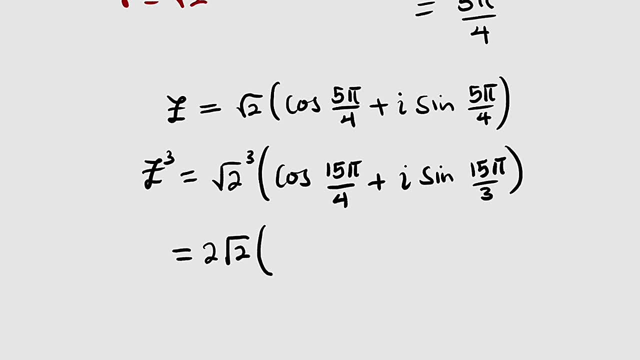 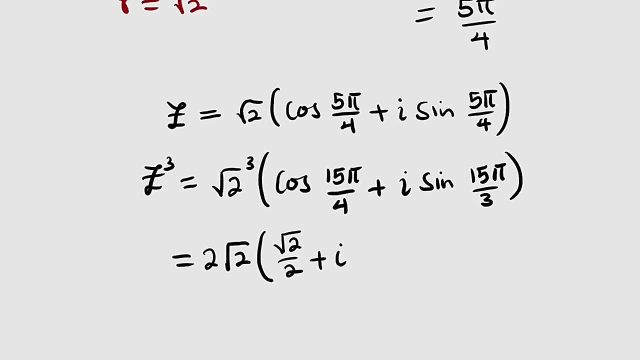 Then multiply by what is cosine of 15 pi divided by 4.. So we have root 2 divided by 2.. Then, plus i, What is sine of 15 pi divided by 4?? All right, sorry, this should be 4, not 3.. 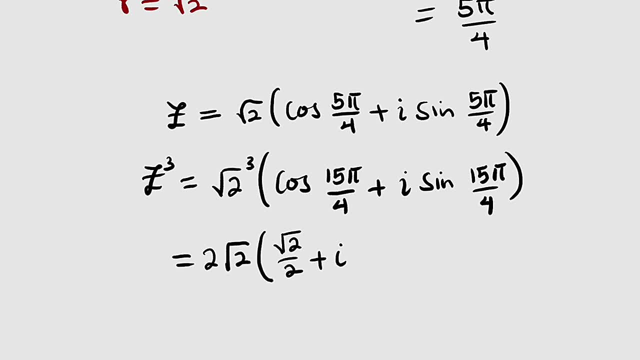 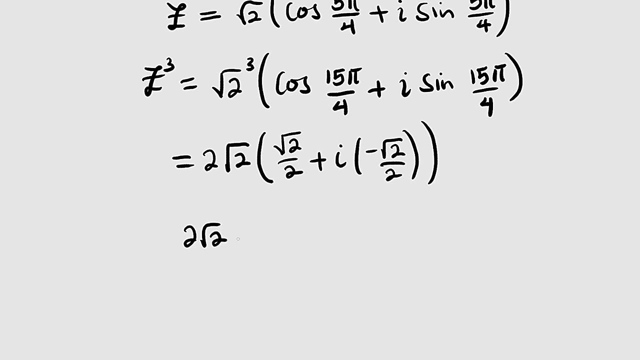 Sine of 15 pi divided by 4 is negative root 2 divided by 2.. So we have negative root 2 divided by 2.. All we have to do is to expand. We have 2 root 2 multiplied by root 2 over 2.. 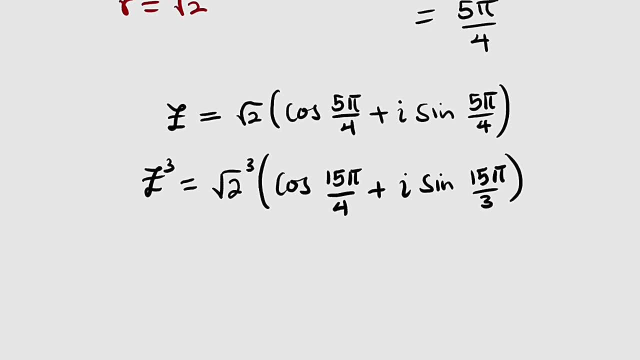 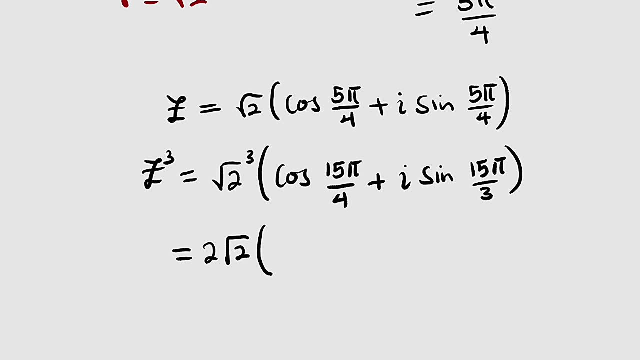 So now let us evaluate this: Square root of 2 to the power of 3 is equal to 2 root 2.. Then multiply by what is cosine of 15 pi divided by 4.. So we have root 2 divided by 2.. Then plus i. 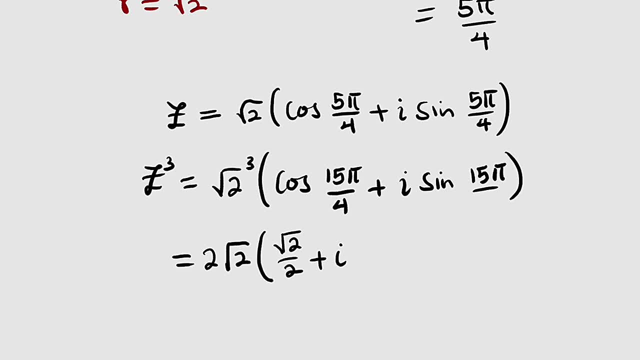 Sine of 15 pi divided by 4.. All right, sorry, this should be 4, not 3.. Sine of 15 pi divided by 4 is negative root 2 divided by 2.. So we have negative root 2 divided by 2.. All we have. 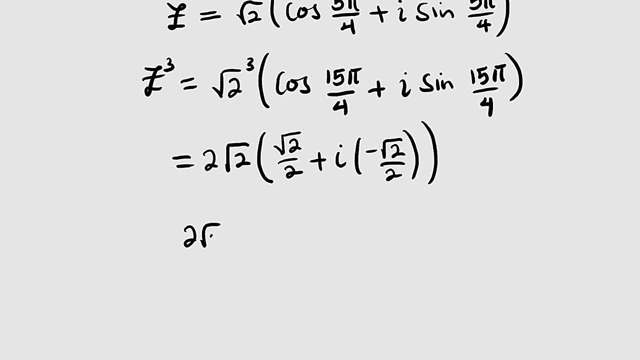 to do is to expand. We have 2 root 2 multiplied by root 2 over 2.. There are minus because of this minus sign. 2 root 2 multiplied by root 2 over 2i 2 will cancel 2. definitely Root 2 times root 2 is. 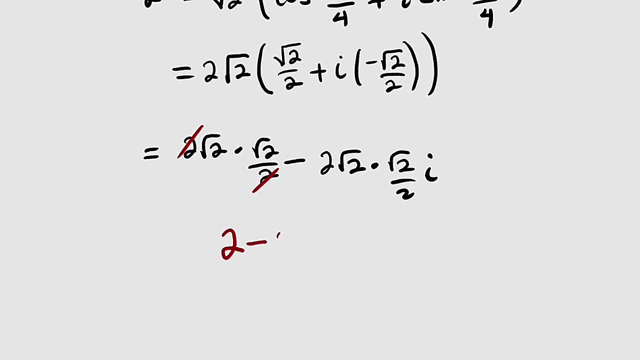 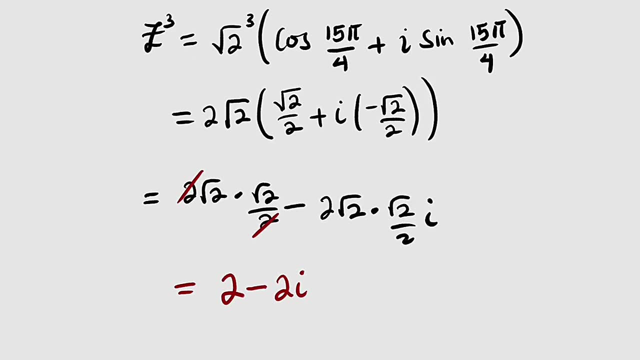 2. So we have 2 here Minus This is also 2i. So after expanding this complex number to the power of 3, we have 2 minus 2i. But remember we have to take the reciprocal Look. 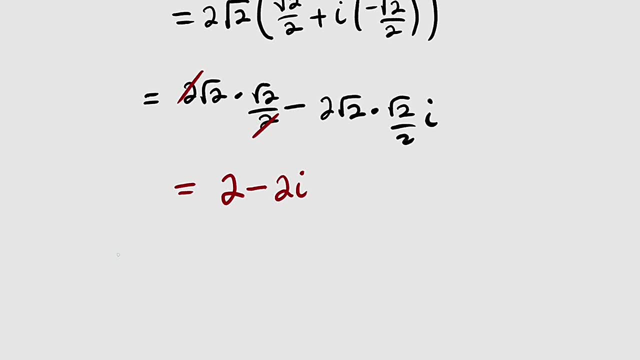 at it here. Move out our haunted square root and multiply it by 2.. Now the multiplier that i took from greater than 2 is equal to what i was giving for little name응. So 1 by r� to the power of 3 is equal to 1 by 2, which Crisisioni gets to 3. And we have 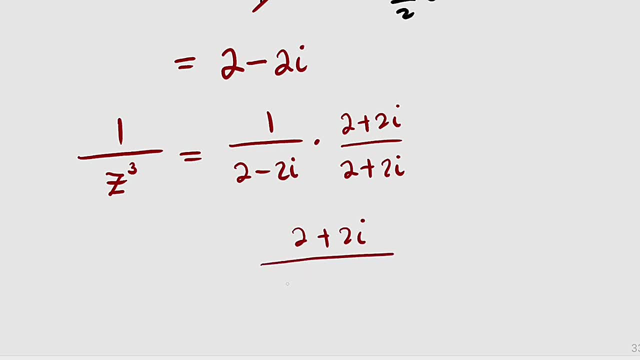 2.. Therefore, 1 divided by our complex number to the power of 3i is equal to 1 divided by 2 minus 2i. So let us multiply the top and the bottom by the conjugate of the denominator which: 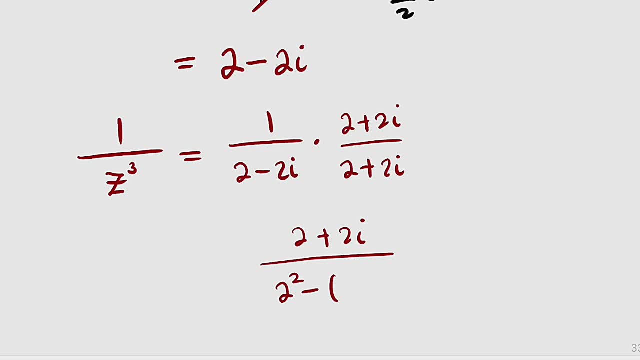 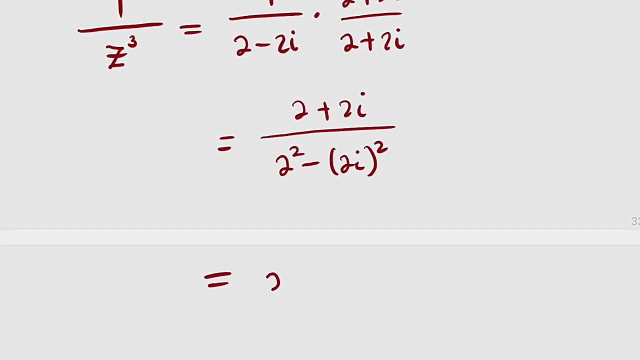 of 2 squared. 2 squared minus 2i, also squared To the top, we have 2 plus 2i. To the bottom, we have 4 minus 2i. squared is 4i squared, but i squared is negative 1.. Therefore, this becomes: 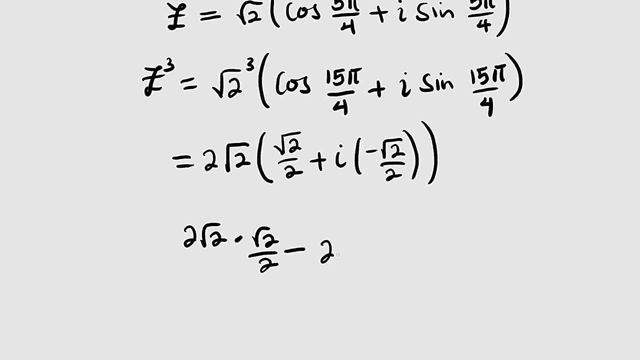 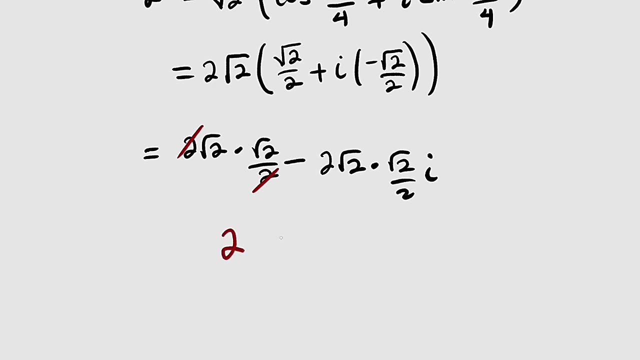 Then minus because of this minus sign: 2 root 2 multiplied by root 2 over 2i. 2 will cancel 2. definitely Root 2 times root 2 is 2.. So we have 2 here. Minus this is also 2i. 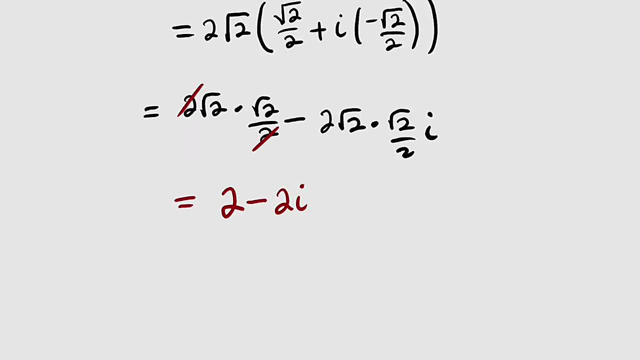 So after expanding this complex number to the power of 3, we have 2 minus 2i. Remember, we have to take the reciprocal look at it here. Therefore, 1 divided by our complex number to the power of 3 is equal to 1 divided by 2 minus 2i. 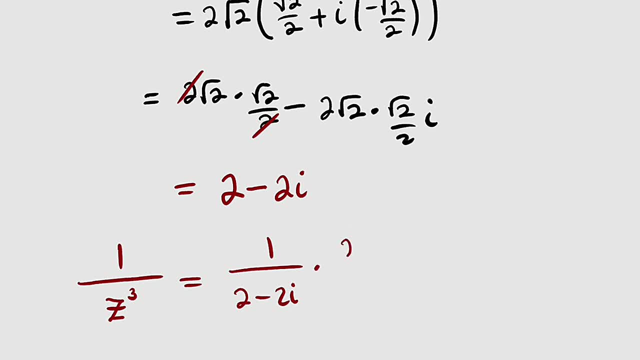 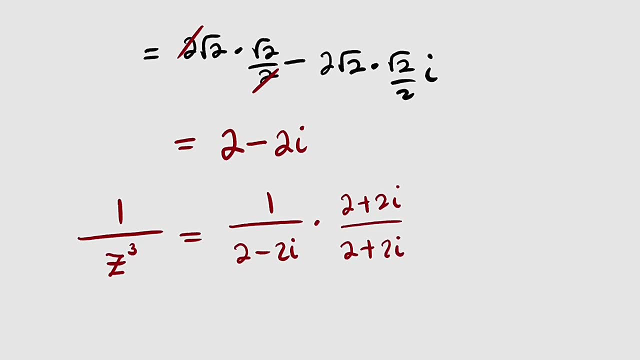 So let us multiply the top and the bottom by the conjugate of the denominator, which is 2 plus 2i. We have to do the same thing here: 2 plus 2i. To the top, we have 2 plus 2i. 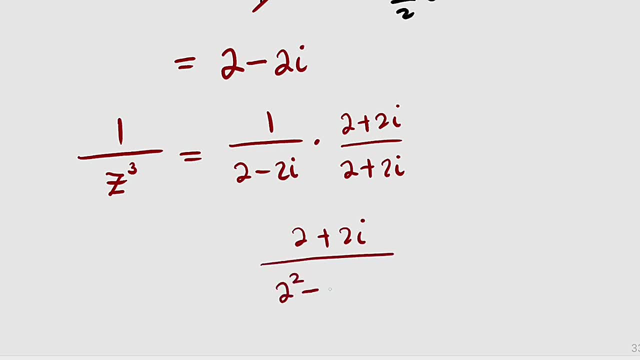 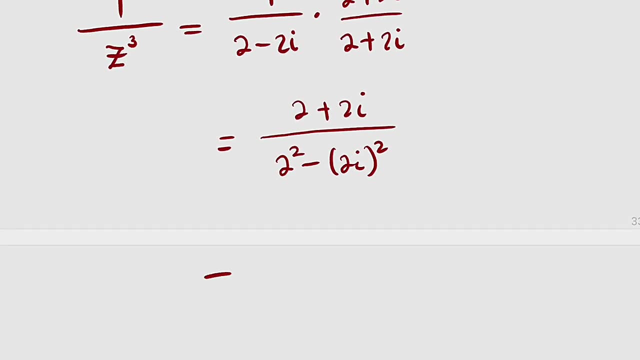 To the bottom, we have difference of 2 squared. 2 squared minus 2i, also squared. To the top, we have 2 plus 2i. To the bottom we have 4 minus 2i. squared is 4i squared. 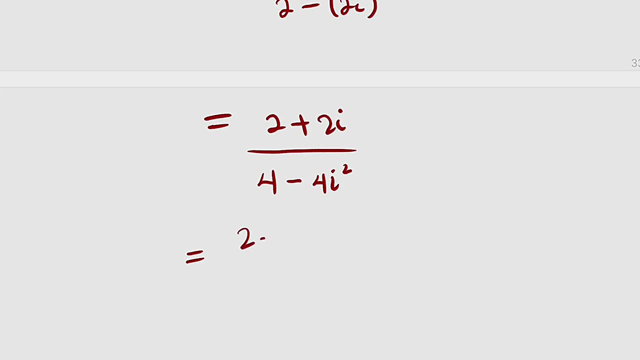 But i squared is negative 1.. Therefore, this becomes 2 plus 2i divided by 4 plus 4, which is 8, right? So this is 2 plus 2i divided by 8, which we can split as 2 divided by 8 plus 2i divided by 8.. 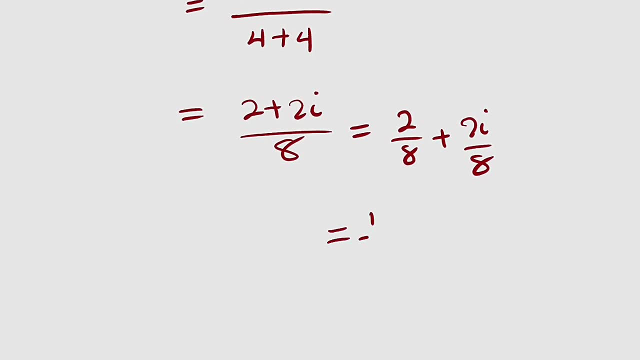 In both cases we have 1 over 4, right? This is equal to 1 over 4 plus 1 over 4.. Therefore, if you expand negative 1, negative i, to the power of negative 3, this is exactly what you are going to obtain. 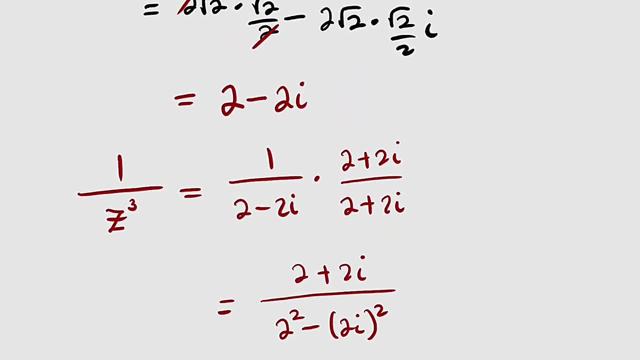 Thank you for watching. Do share to your learning colleagues And don't forget to subscribe to my YouTube channel for more exciting videos. Bye, bye.